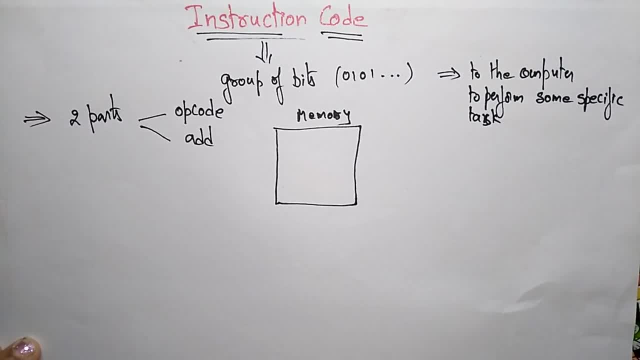 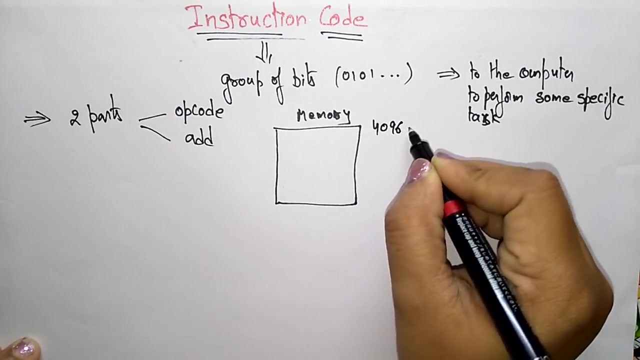 getting the instruction code and that we are going to be converted into group of bits and that group of bits will remain under the instruction code. we are coming up with the instruction code and that group of bits, which is the novell departure能, will be read by the processor. So actually this memory will be the size of 4096 x 16.. 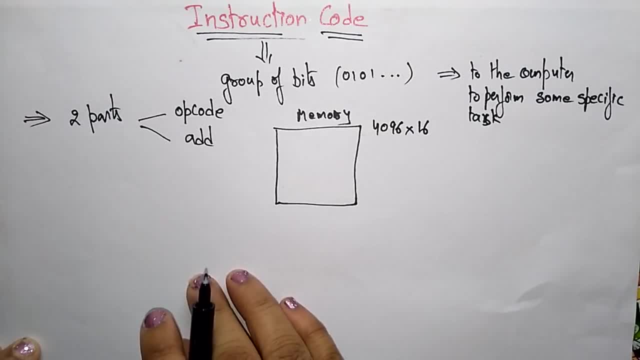 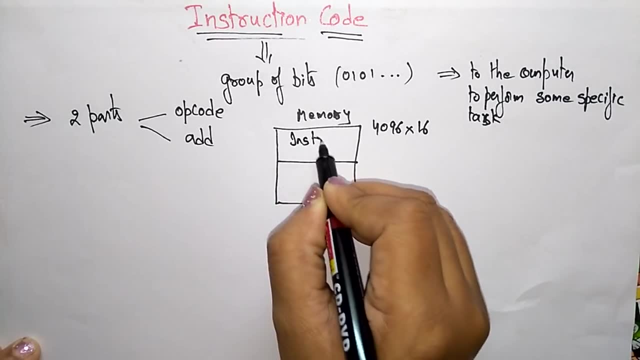 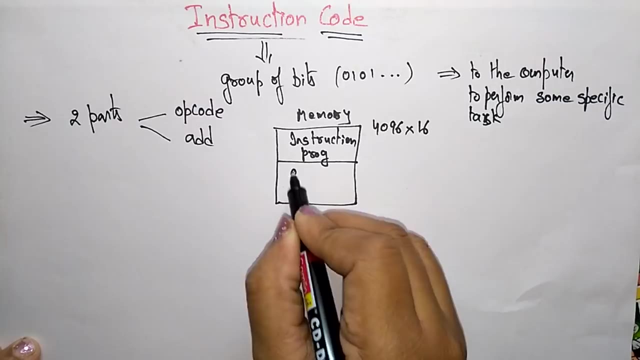 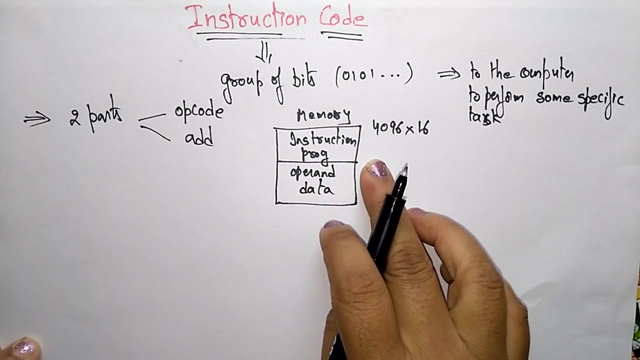 So this is the size of the memory for the 16 bit instructions. So this memory will be divided into two parts. So one holds the instruction program, instruction program- and another will holds the operand, that is, the data. So memory is having instruction program and then is: 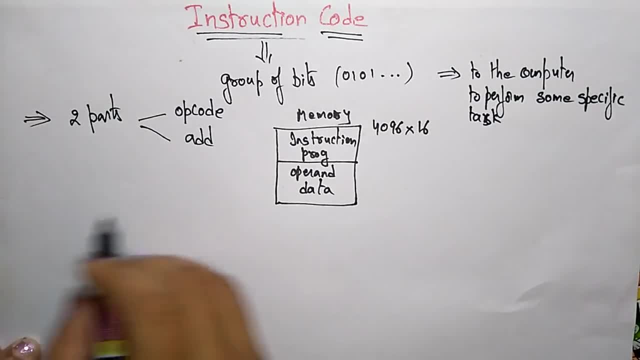 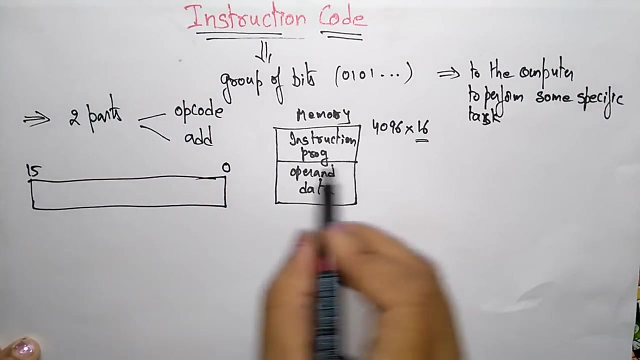 operand data. So here actually this instruction code is of size 16 bit because it is having 4096 x 16 memory location. So this instruction code format will be divided. It is a 16 bit address from 0 to 15.. So in this 0 to 15,, 4096 means this is a 2 power, 12 and 16 means 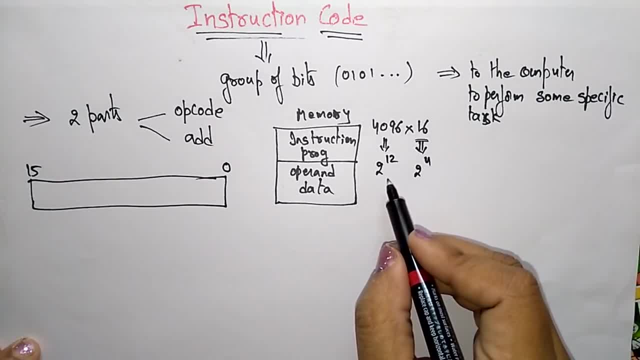 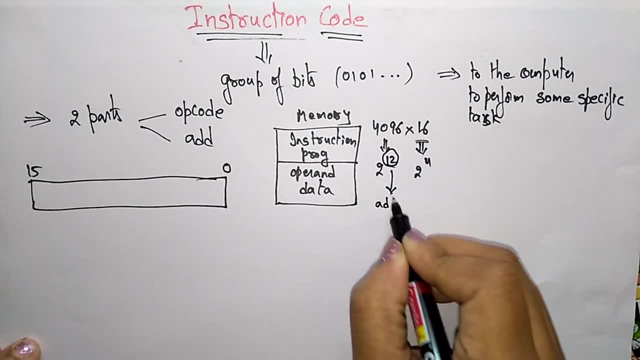 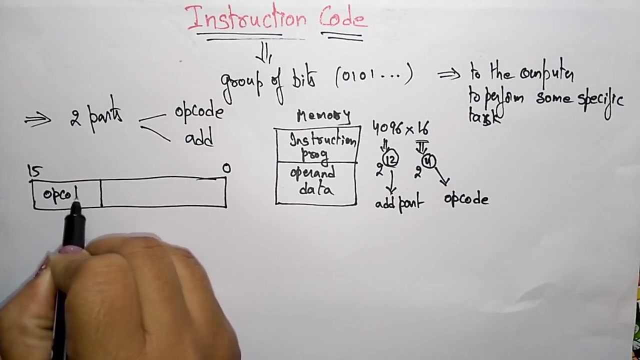 2, power 4. Means: here the 12 bits specifies the. this 12 bits specifies the address part and this 4 bits specifies the opcode. So the instruction code will be divided into two parts. One is address part and another is opcode. So here the 4 bits will specifies the opcode 0 to sorry, 15 to 12.. And the: 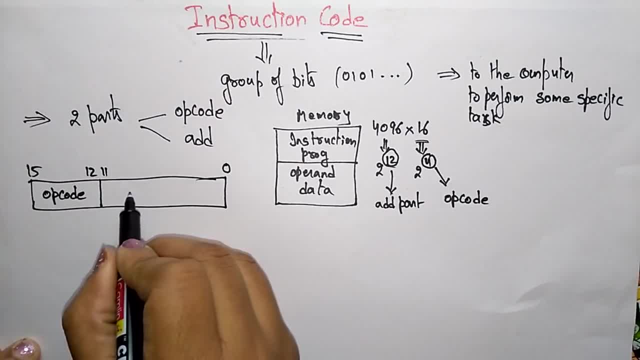 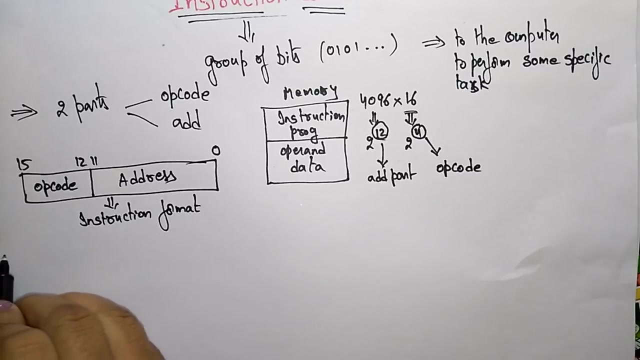 remaining 12 bits, 0 to 11, will specifies the address part. So this is the instruction format. This is the instruction format. So actually this instruction is of three types. It's a memory reference instruction, register reference instruction. memory reference instruction. 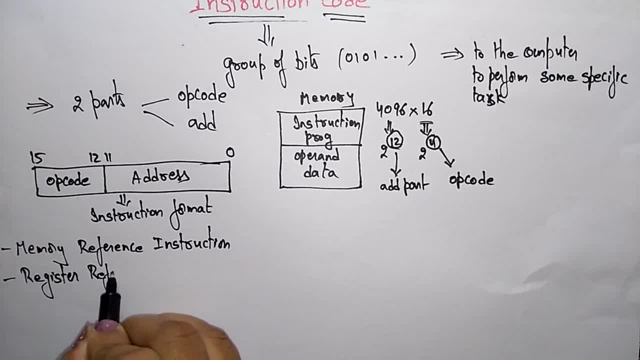 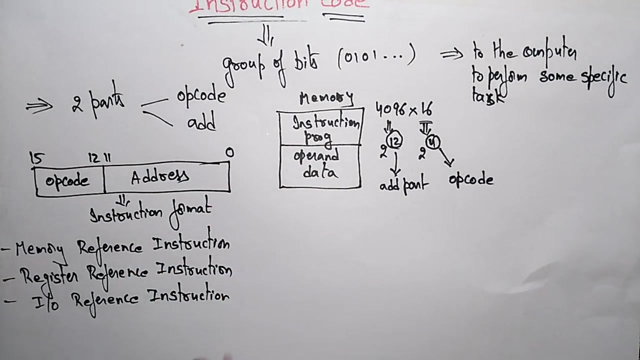 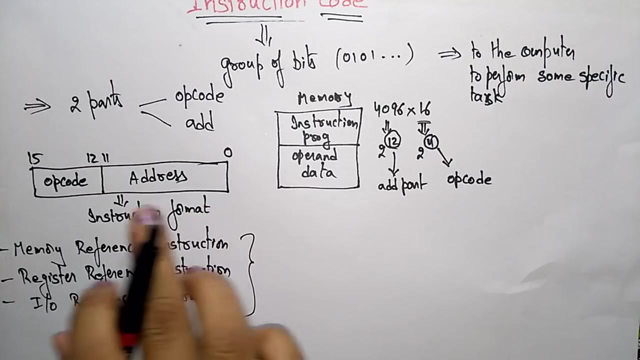 or Ivo reference instruction. So this instruction which we are getting from memory, or we can get from a register, or it is our Ivo. So whatever the instruction that will be is of is of three types: Memory reference instruction, or it is a register reference instruction, or it is a Ivo reference. 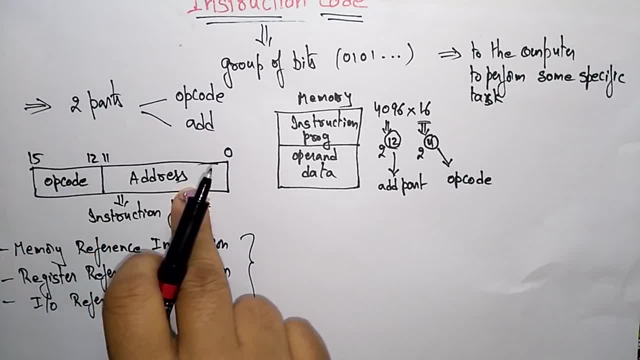 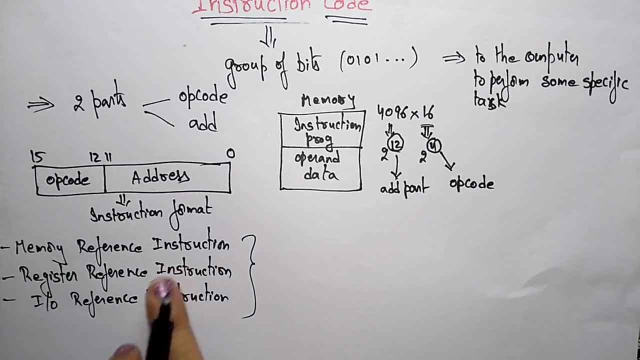 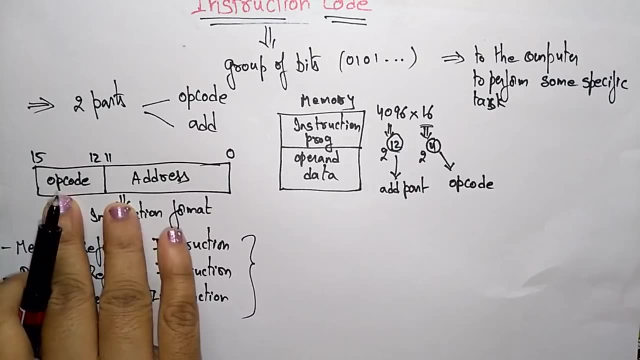 instruction. So, based on this instruction, the browser will understand what type of instruction we are getting. So this instruction is coming from memory reference, or it is from register reference, or it is from Ivo reference. Okay, So actually this instruction code can be of: 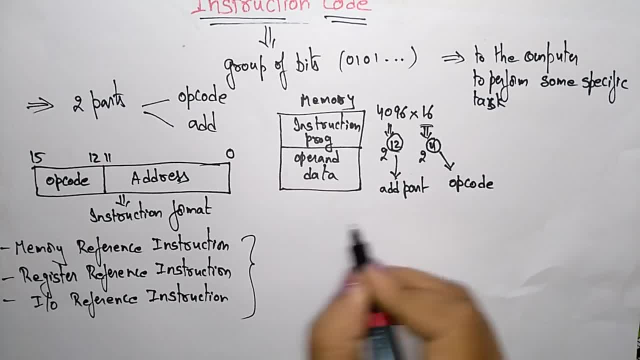 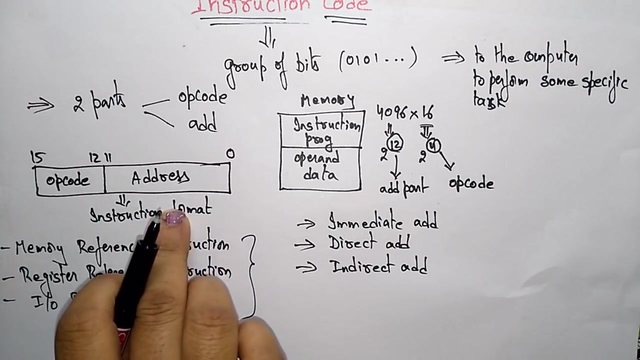 three types And it is in the format of like immediate address, direct address, indirect address. So this instruction holds opcode and address. So this opcode and address will be of immediate or direct or indirect. So, based on the instruction, the processor can understand. the instruction which it gets is whether it is immediate data, or it is a direct data, or it is an indirect data. 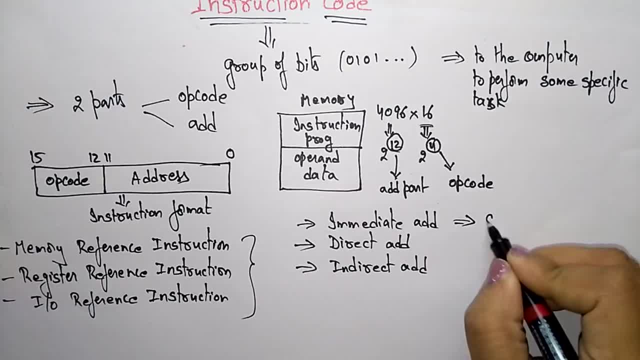 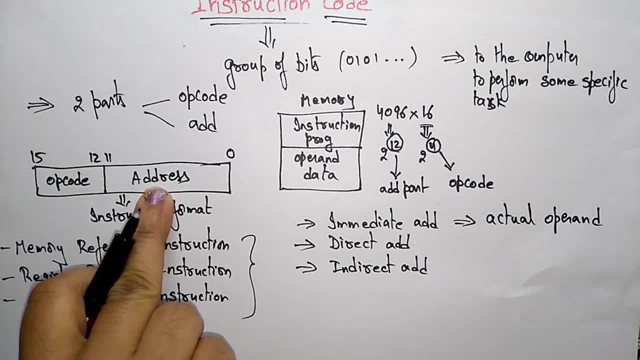 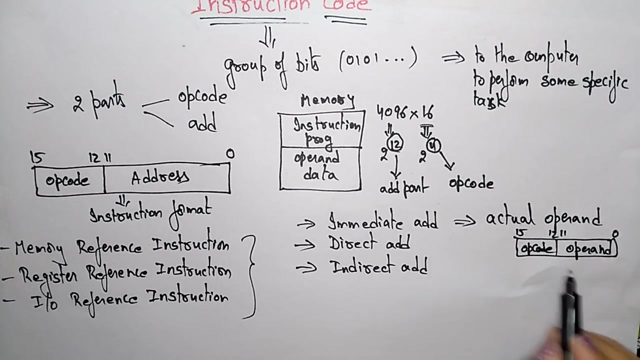 Immediate means. it specifies actual operand. So actual operand will be present in the immediate address means: opcode. So this is 0 to 11,, 12 to 15.. So this is the immediate address, opcode and operand- direct operand- will be present. 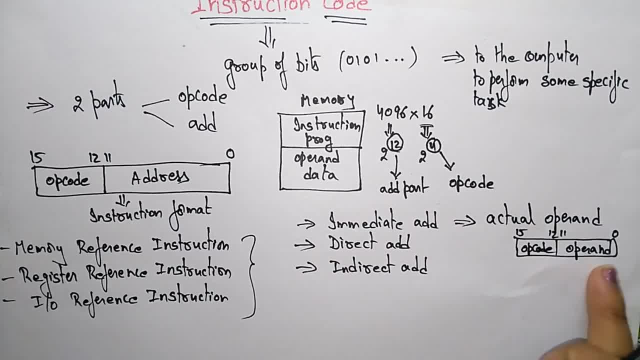 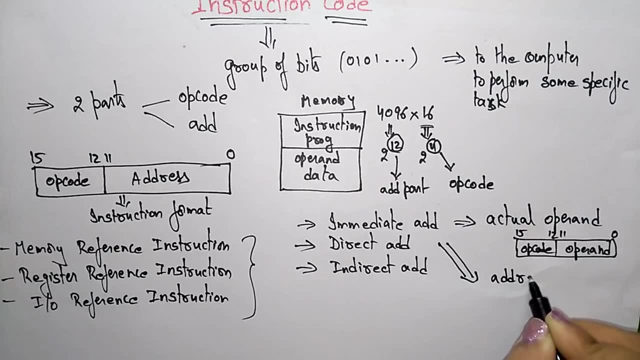 So then the processor understand this is an immediate address, So we are just getting the operand and it calculates the operation. Now coming to the direct address, So what this direct address specifies? Direct address specifies the operation. Address of operand. Address of operand. 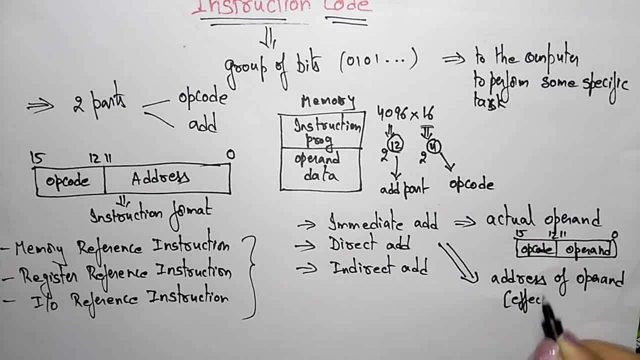 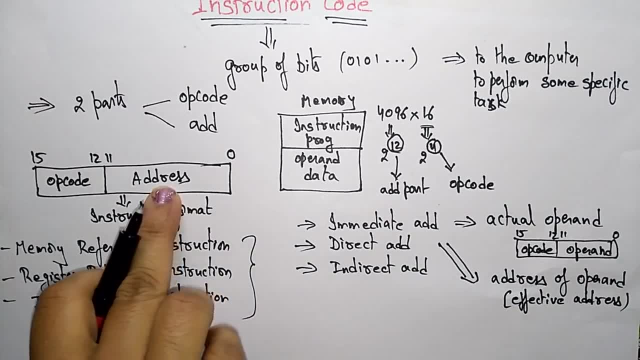 So we call it as an effective address. Effective address, So direct address, holds the address of the operand Here in this place, 0 to 11, if address of the operand is present then we call it as a direct address. Means just suppose this is a memory location. 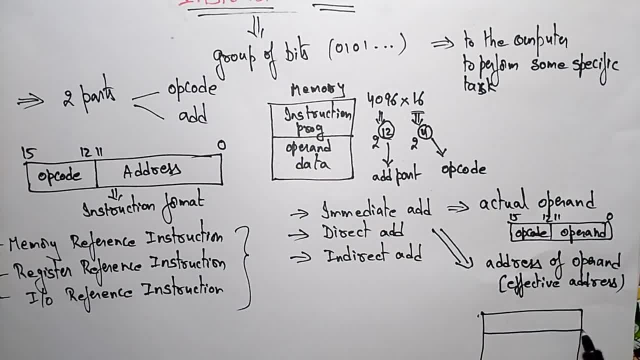 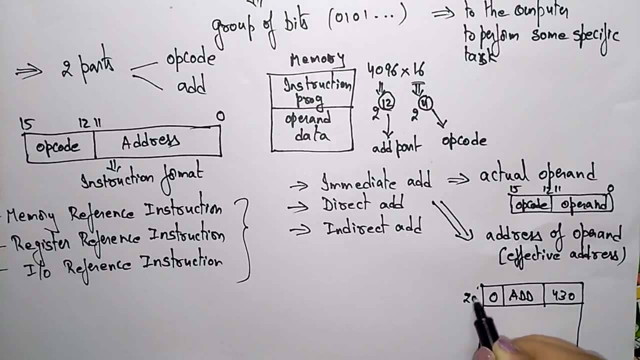 So which I said here, This is an instruction program. Instruction will be present, So this instruction may be suppose add. So it was 430.. This is some memory location. So in the particular 430, you are having the actual operand. 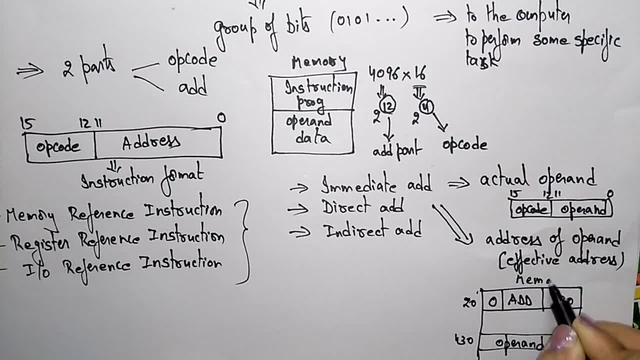 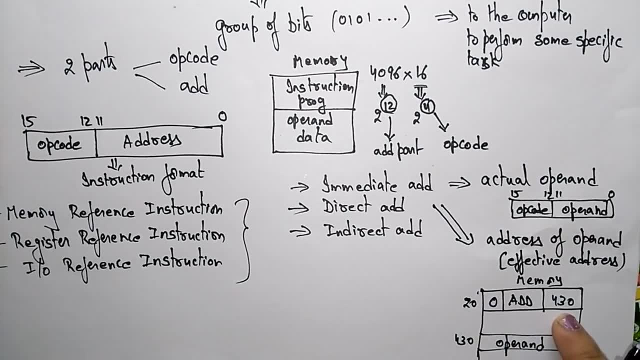 Actual data will be present. So this is the memory location. So in that memory location The instruction will be like this: 0 at 430.. 430 here indicates the address of operand. So this is the address of operand. So where this address, in this 430 location, you are having the operand. 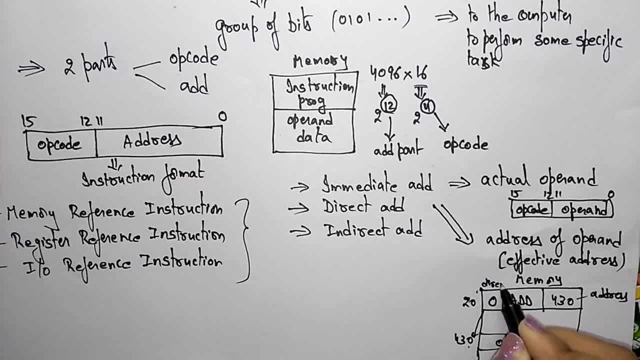 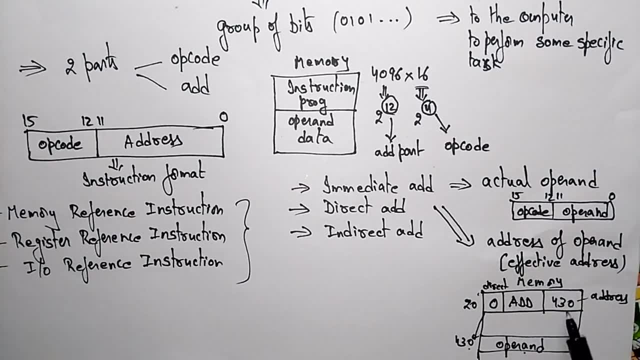 So here the 0 indicates it is a direct address. So this is direct. So in that particular address of operand in this 430 is address In that particular address location you are having the operand. This is the effective address. You call this as direct addressing. 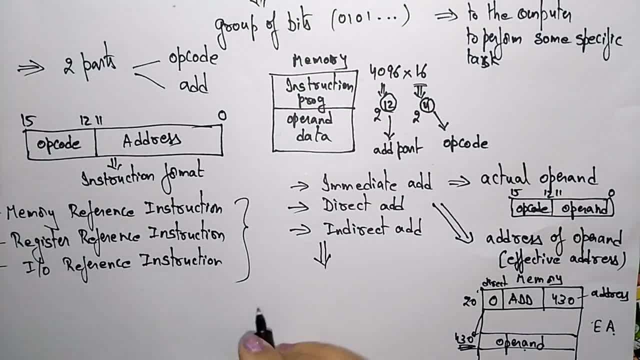 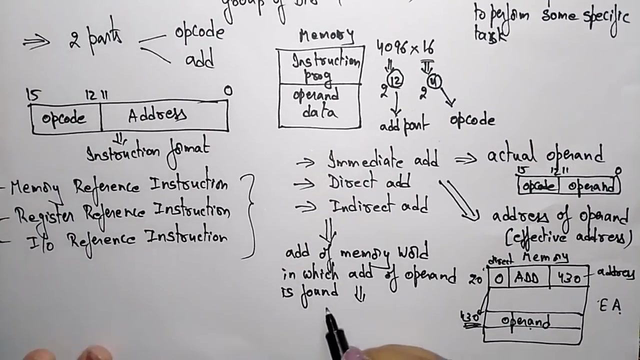 Now coming to indirect addressing. Indirect addressing specifies the address of memory word. So it specifies the address of memory word In which address of operand is found. so first it holds the address of memory word. in that particular address of memory word, address of operand is present. again, you have to go to that particular operand. so it's look like this: 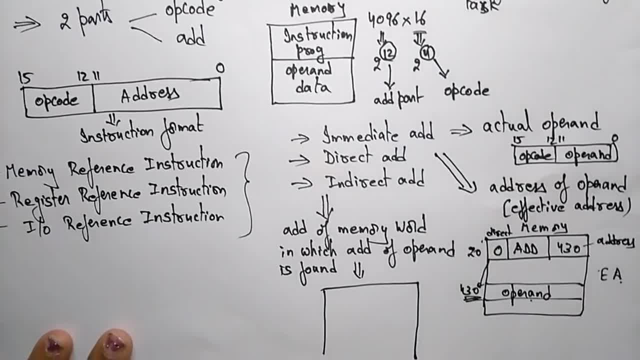 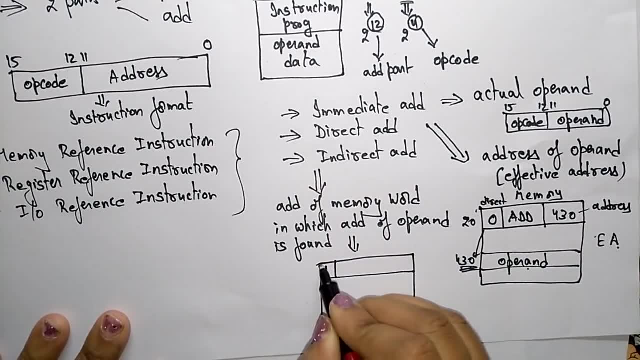 so this is the memory location. so but if it is an indirect addressing you have to keep it as 15th bit is the i1 at 430, 20. so in that particular 430 location you are having the address of the operand. so again you have to go to that particular address.